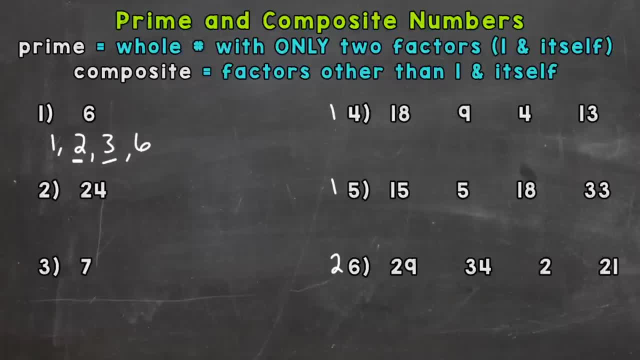 than one and itself. We have a two and a three here as well, So it's automatically composite. A prime number will only have one and itself as the factors. Number two: twenty-four- Well, we know one and twenty-four, And twenty-four actually has a lot of factors. 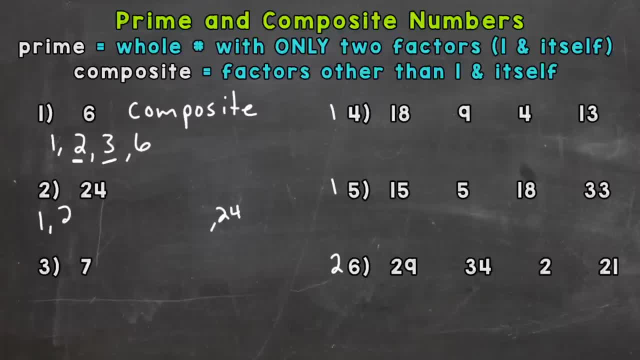 or numbers that can multiply to get twenty-four. So we know two and twelve can multiply to get twenty-four. Three and eight and four and six. So we have a lot of different factors there for twenty-four. So this one is easily composite. 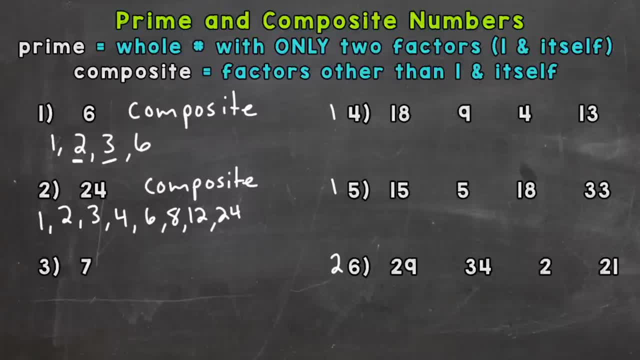 Number three, seven. So let's think of the factors of seven. Which, which multiplication facts or numbers can we multiply together to give us seven? And actually it's only one in seven, One times seven or seven times one. So this only has two factors, one and itself. So seven is prime. 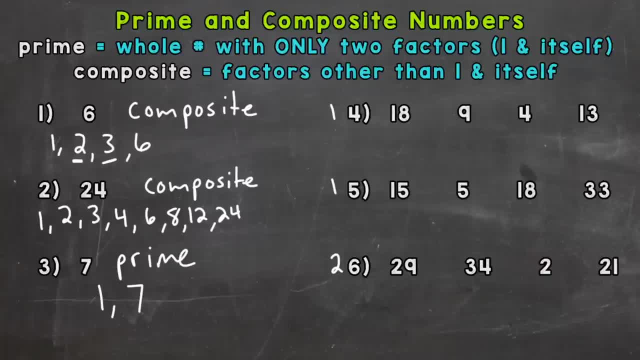 Number four. let's go through all four choices and find the prime number, So eighteen. well, this is even and we automatically know that two can go into all of the numbers, can go into all even numbers. So all even numbers, except for one special one, are going to be: 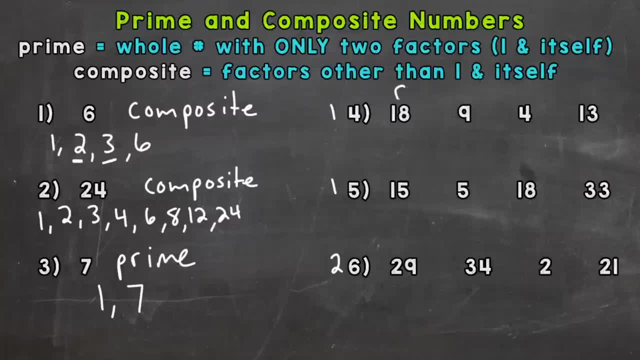 composite, So 18 is composite. I'll put a C here because we know 1 times 18,, 2 times 9,, 3 times 6.. So we have a lot of different factors there. So composite 9, well, 1 times 9 is 9, and we can also. 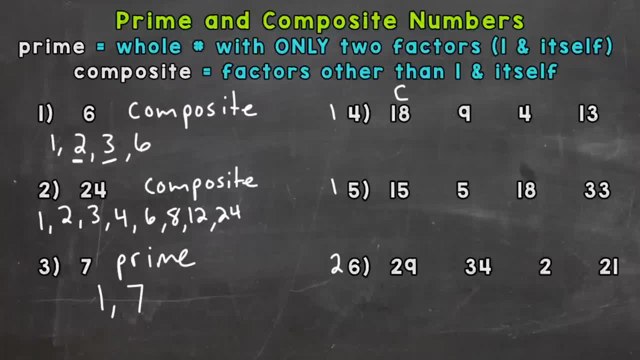 do 3 times 3.. So we have three factors for 9, and that means it's composite because it's more than 1, and itself. Now a common misconception when people start looking at prime and composite numbers for the first time, are thinking that all evens are composite and then all odds are. 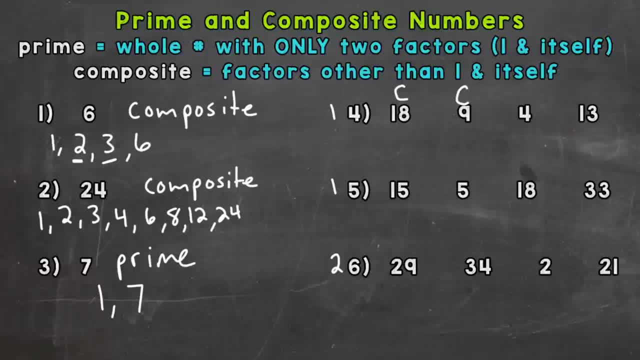 automatically prime, which isn't true. Odd numbers can be composite, just like this: 9 here, 4, well, 1 and 4. and then also 2, 2 times 2, right. So 4 is composite. And then the last one, this is: 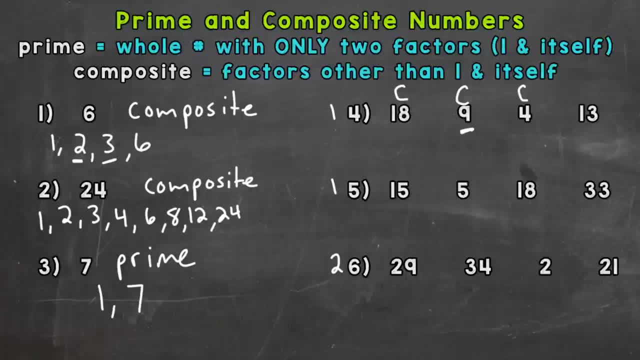 going to be our prime number. The only numbers, only factors of 13, are 1 and 13.. So 13 is our prime number there. Let's take a look at number 5.. 15, again, don't just think, because it's odd. 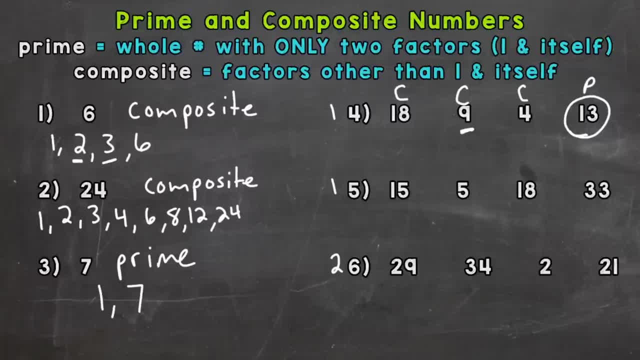 that it's composite. It's composite. So let's take a look at number 5.. 15, again, don't just think, because it's odd, that it's composite. It's going to be a prime number. 1 and 15, also 3 and 5 are. 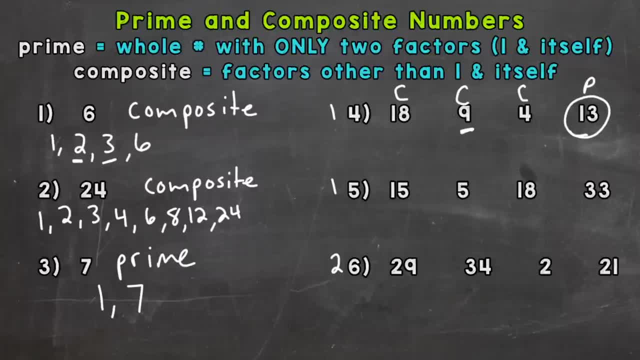 factors: 5 times 3 or 3 times 5 equals 15.. So 15 is composite, Now 5. on the other hand, the only factors of 5 are 1 and 5.. So 5 is prime 18, composite 33 almost seems like it would be prime. 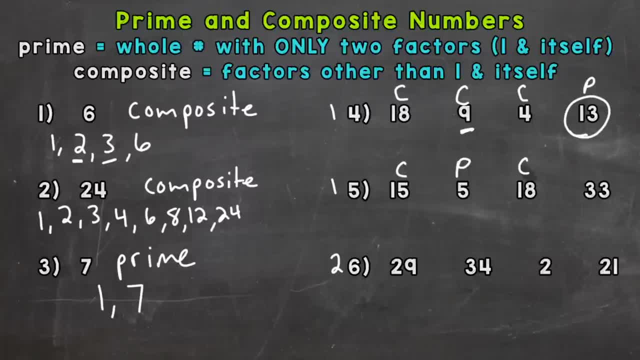 1 and 33,. but we can divide 33 by 3 and get 11.. Or think of our multiplication facts: 3 times 11 equals 33.. So 33 is composite And number 6,. we have two prime numbers here, The first one being 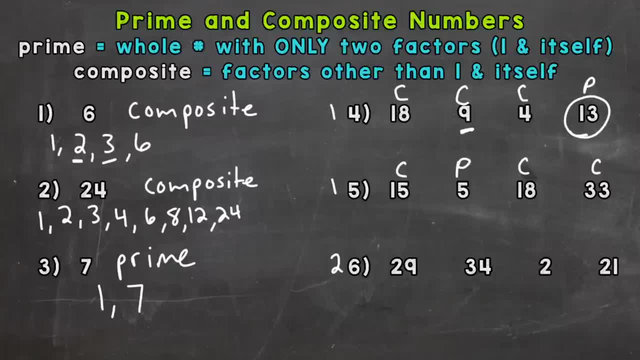 this 29.. The only factors of 29 are 1 and 29. So we have a prime number here. 34 is even, So we know that it's going to have more than just 1 and itself. So we have 1,, 34,, 2, and 17.. So 34 is composite. Next we have 2,, which is kind of a 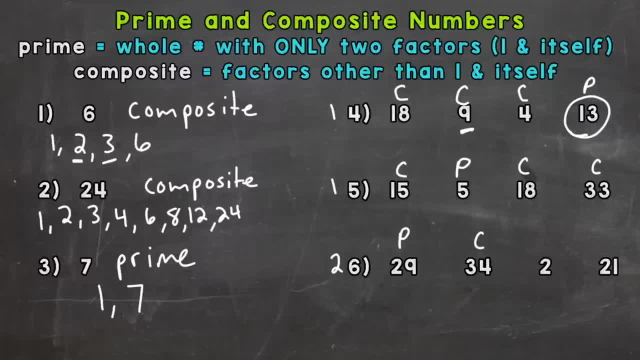 special number here, because it's the only even number that's prime. 2 only has two factors: 1 and itself, 1 and 2.. So again 2, the only even number that is actually prime. Then we have 21..